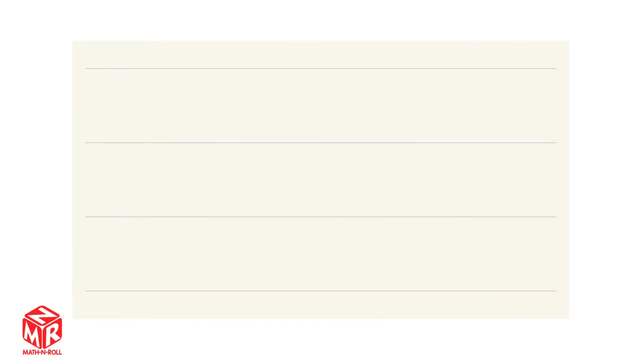 Let's try another example: 6 plus an unknown number equals 13.. To find the missing number, we take the whole 13, and subtract the part that we know, 6.. So 13 minus 6 equals 7.. 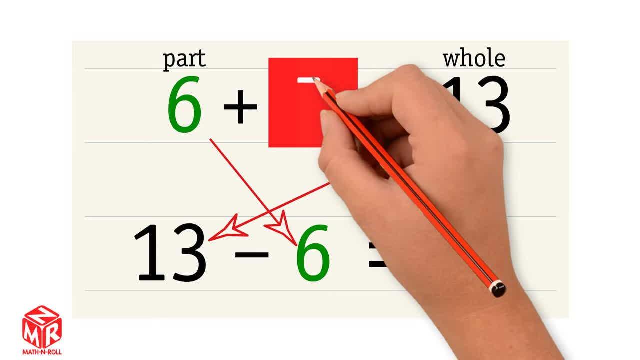 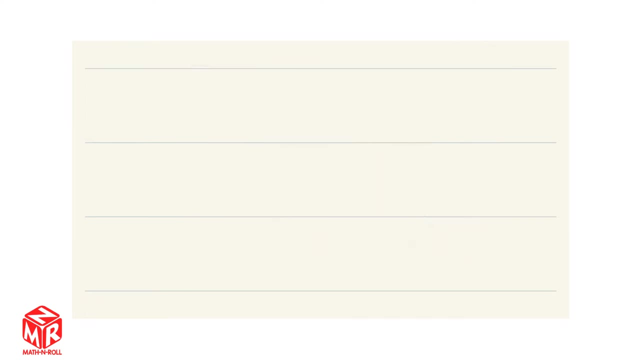 7 is the unknown number. 6 plus 7 equals 13 and 13 minus 6 equals 7 are related facts. We use related facts to find unknown numbers. Let's try another example: 9 plus an unknown number equals 15.. We can find the unknown number by taking the whole 15, and subtracting. the part that we know: 9.. 9 plus 7 equals 11.. 9 plus 7 equals 15.. 9 is the unknown number. 7 is the unknown number. 7 is the unknown number. 9 plus 7 equals 13.. 9 minus 6 equals. 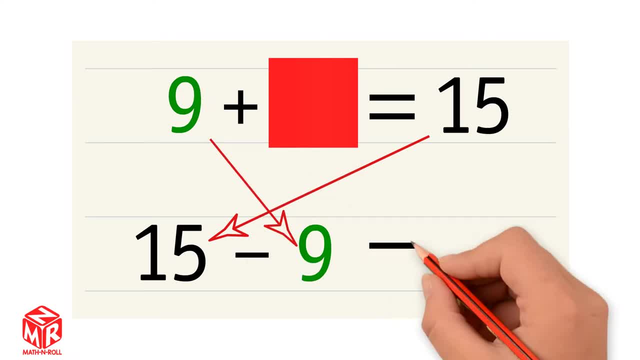 15 minus 9 equals 6.. So 6 is our unknown number. 9 plus 6 equals 15, and 15 minus 9 equals 6 are related facts. Let's try another one: An unknown number plus 5 equals 14.. 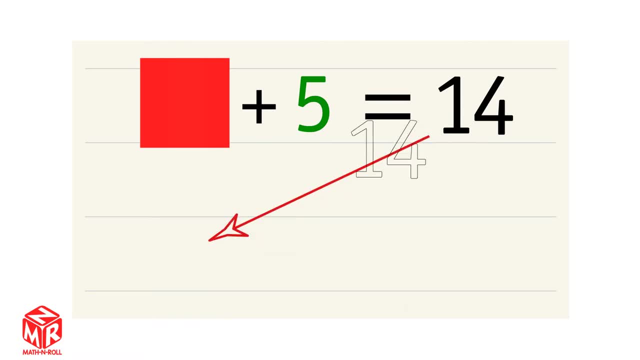 To find the unknown number, we take the whole 14, and subtract the part that we know, 5.. 14 minus 5 equals 9.. So 9 is our unknown number. 9 plus 5 equals 14, and 14 minus 5 equals 9 are related facts. 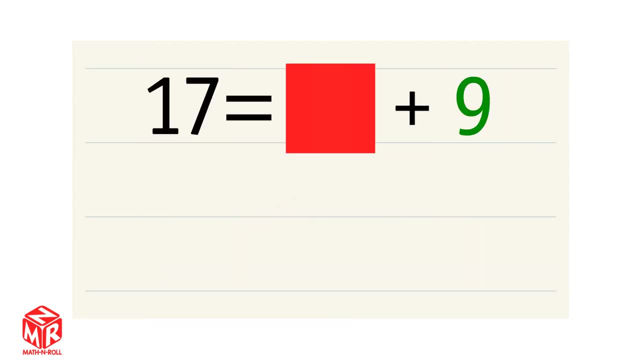 Let's try another one. 17 equals an unknown number plus 9.. To find the unknown number, we take the whole 17, and subtract the part that we know 9.. 17 minus 9 equals 8.. So 8 is our unknown number. 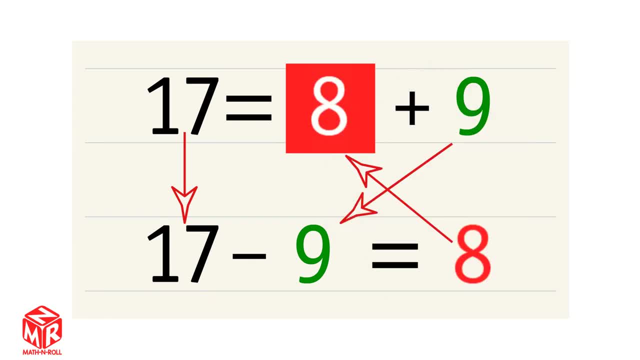 17 equals 8 plus 9, and 17 minus 9 equals 8, are related facts. So to find the unknown number, you take the whole and subtract the part that you know. If you thought this video was helpful, please leave a like. For more videos like this, please subscribe.